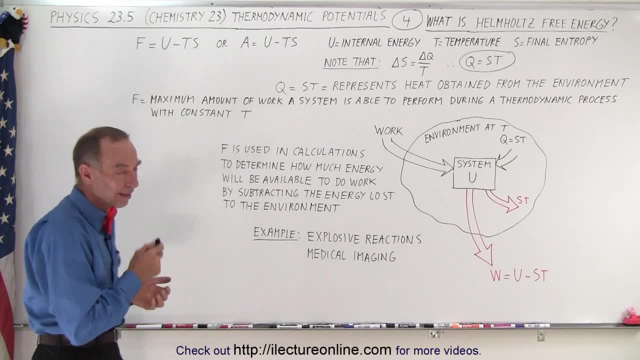 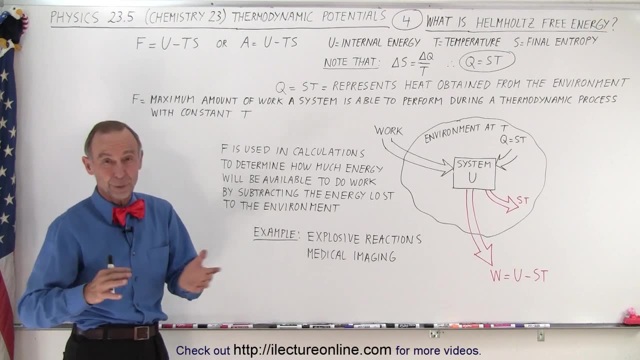 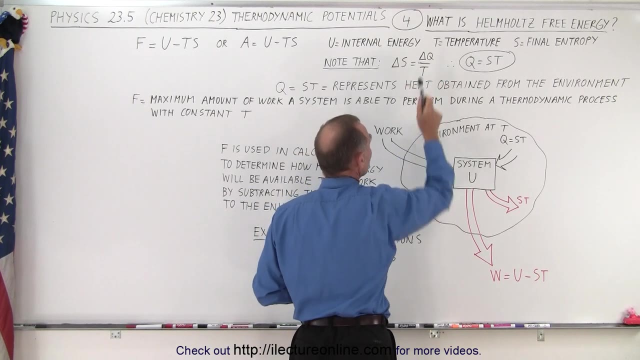 But what is T and S? Well, T stands for temperature and S stands for entropy. Now, without going into too much detail of what entropy is, the equation for the change in entropy is equal to the heat added or subtracted, And I put the little delta symbol in front. 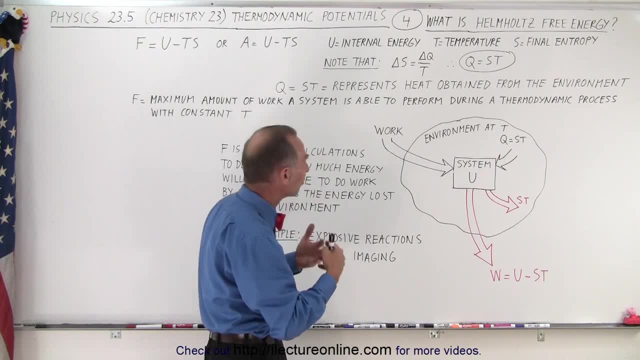 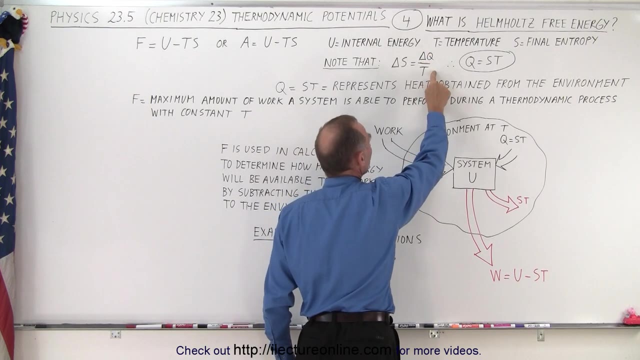 I put it on the Q to make it a little bit more sensible. We don't need to write it, because Q simply represents the amount of heat added or subtracted or taken away from the system. But here we can see that the change in entropy is equal to the ratio of how much heat was exchanged, divided by the temperature at which this happens. 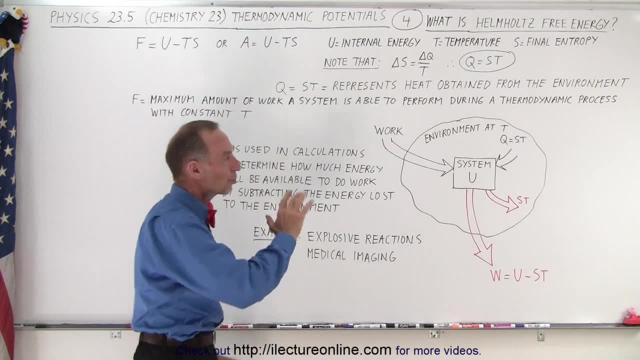 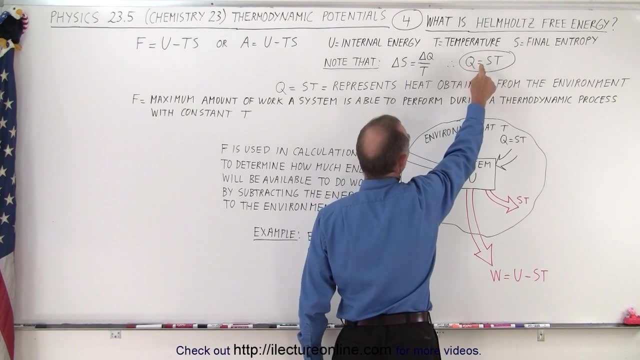 Now, with the Helmholtz free energy, we're going to keep the temperature of the environment the same. It's going to be a constant. So here we can see, then, that we can write Q as simply the product of entropy times, T. 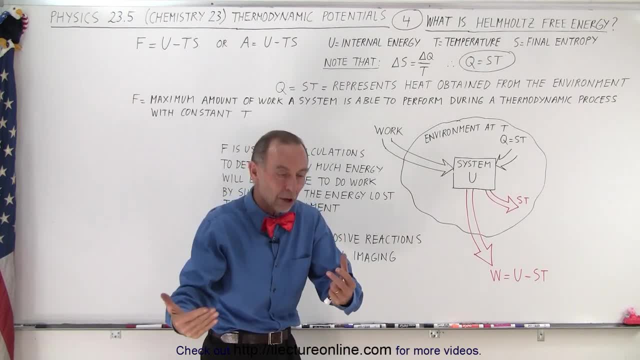 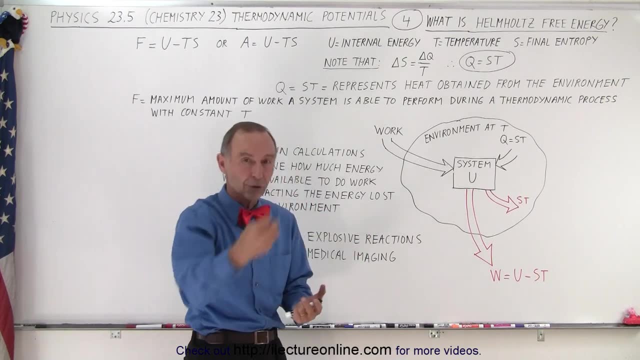 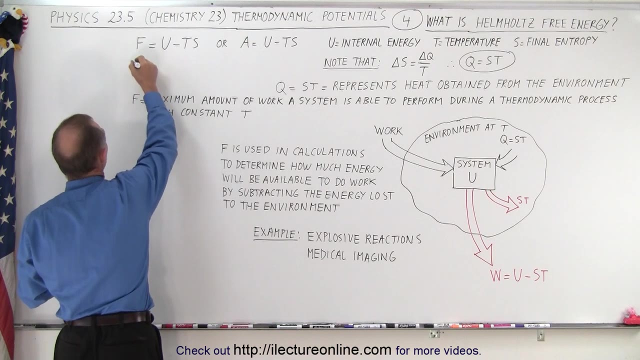 What that really means is that S times T really represents an exchange of heat either from the environment to the system or from the system to the environment. So, even though it seems kind of mysterious, this could really be written as such. We could say: F equals U minus Q. 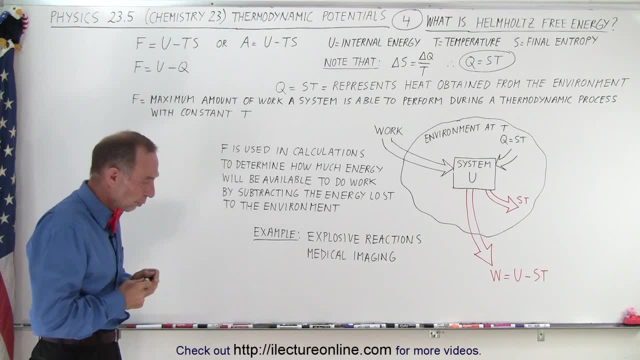 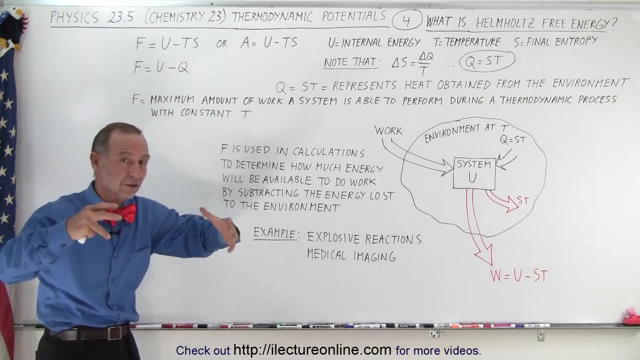 And we know what Q means. Q means heat. So therefore, it's not as complicated, not as mysterious. It simply means that we take all the available internal energy and subtract from that Q. And what does that Q represent? Well, let's come over here to the diagram. 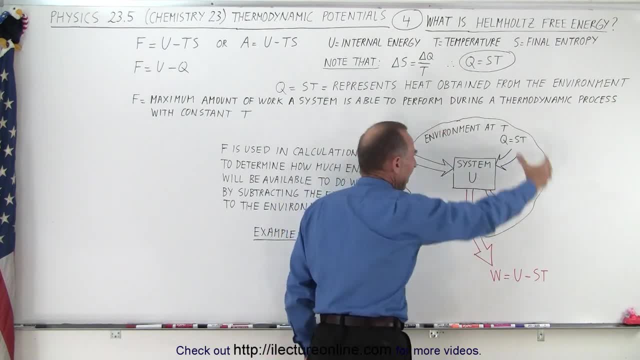 So here we have a system that's enveloped by an environment And the environment is kept at a constant temperature, T, And to change the system we can put some work into the system. When we do work onto the system, it adds energy to the system: internal energy. 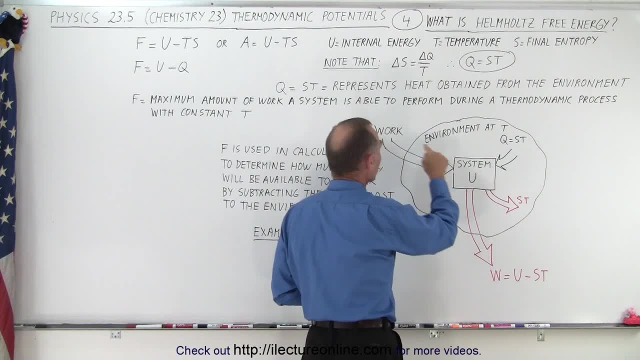 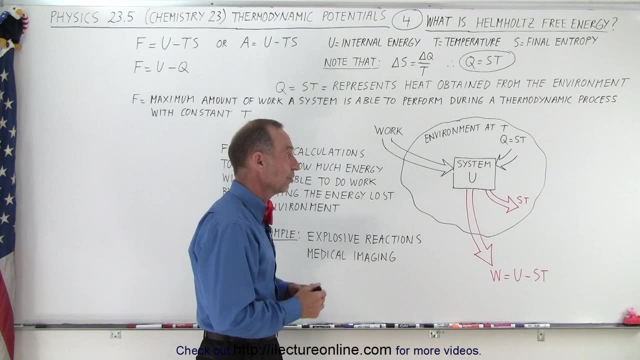 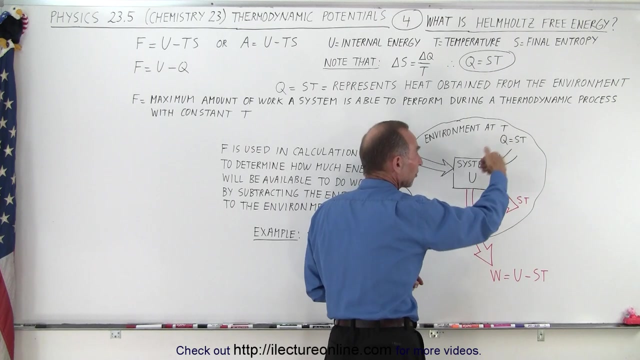 But not all of the internal energy of the system can come from doing work on it. Some of it can be absorbed from the environment at temperature T And so that absorption of energy from the environment into the system, we can call it Q. When Q is positive we add heat to the system. 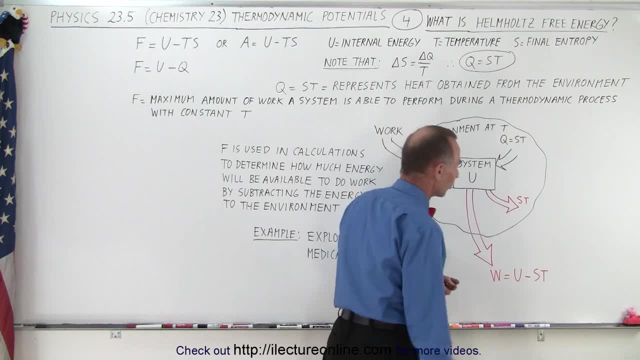 And it's a product of the entropy times. the temperature, Even if you don't understand why or why that's there, that's fine. simply think of it as heat added to the system as well as work done on the system together adds to the internal energy of the system. 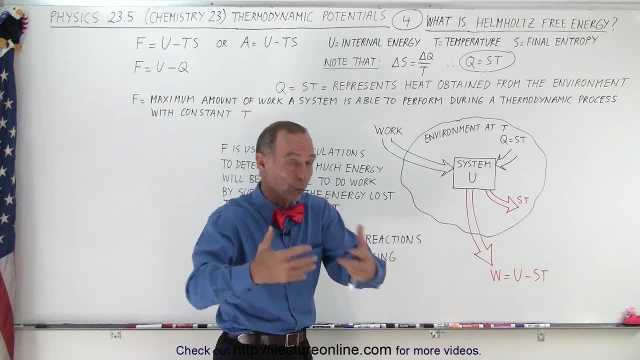 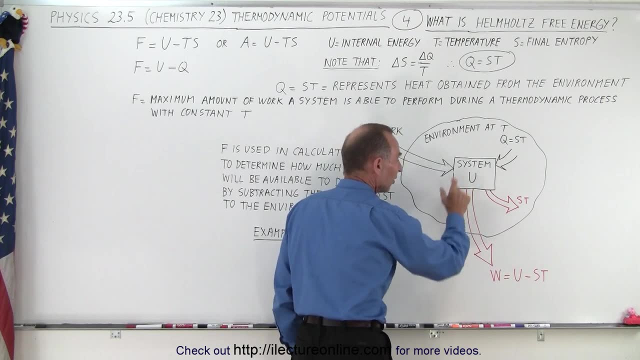 Now, when the system wants to release that energy to do work, well, not all of it will be available to do work, only some of it. So whatever the internal energy is minus, whatever energy goes back into the environment, Again, that's that Q or the ST of that equation. 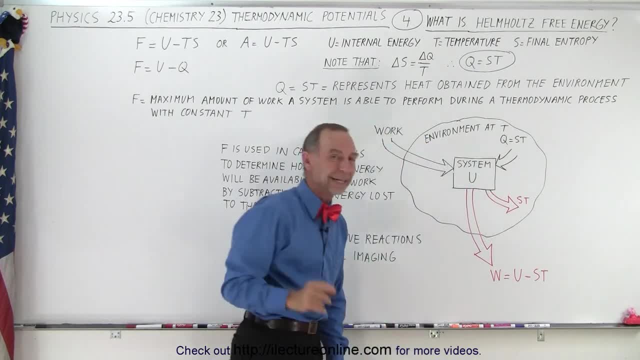 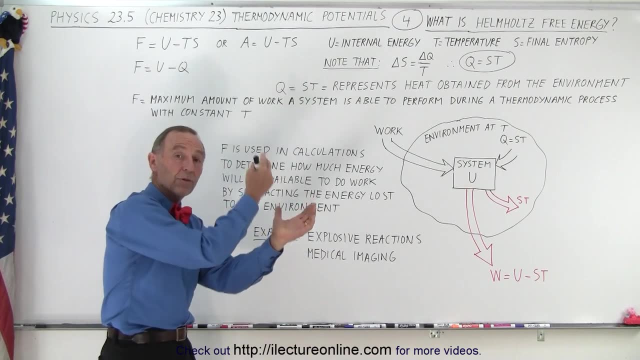 When the system tries to do work, not all of it is available, And that's the key to the Helmholtz free energy. When the system does work, not all of the internal energy is available. Some of it is lost to the environment. 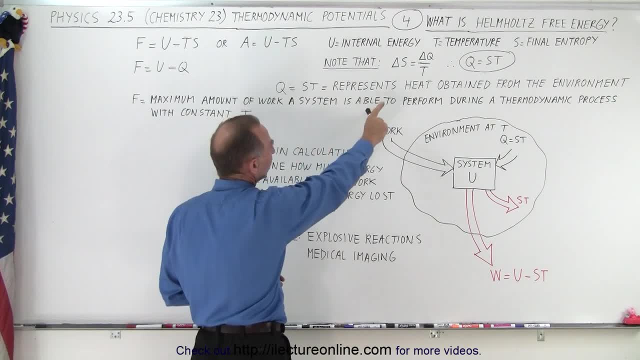 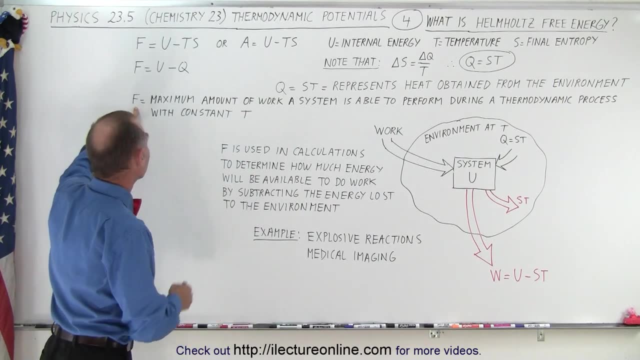 And so we can say that Q here represents the heat obtained from the environment, And of course it also represents the heat returned back to the environment, And therefore we can write that the Helmholtz free energy is the maximum amount of work a system is able to perform. 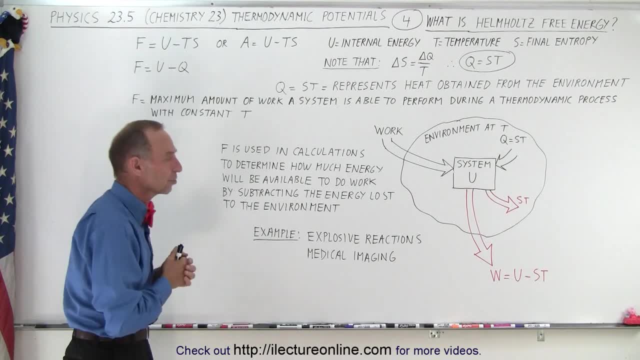 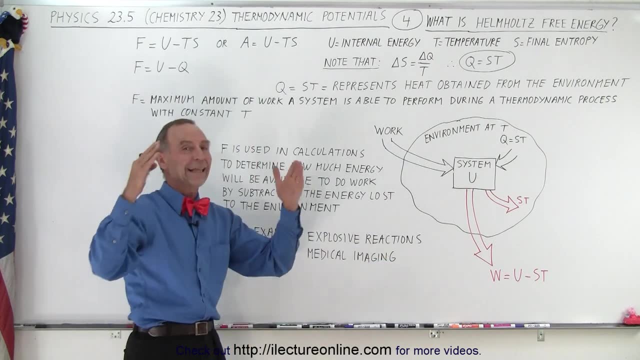 in a thermodynamic process at a constant or with a constant temperature. T In other words. take the internal energy of the system, subtract from it what's going to be lost to the environment, and that's the maximum you can get out of that system. 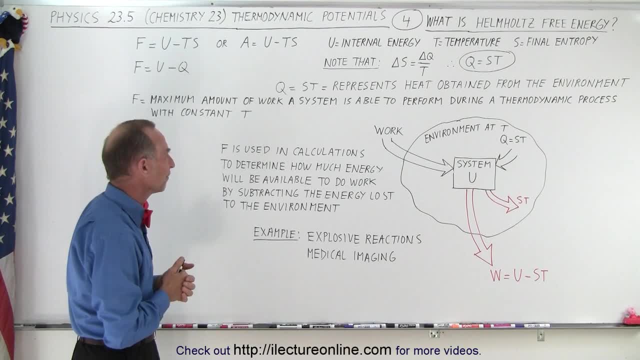 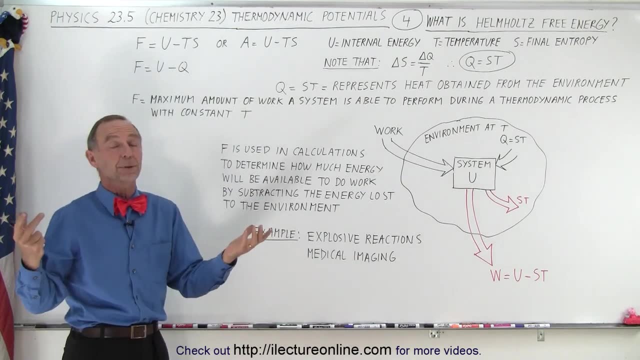 And that's what we mean by the Helmholtz free energy. Now, what do we use it for? Well, it's used in calculations to determine how much energy is available. It's a good thing to know because when we have some sort of reaction or process, 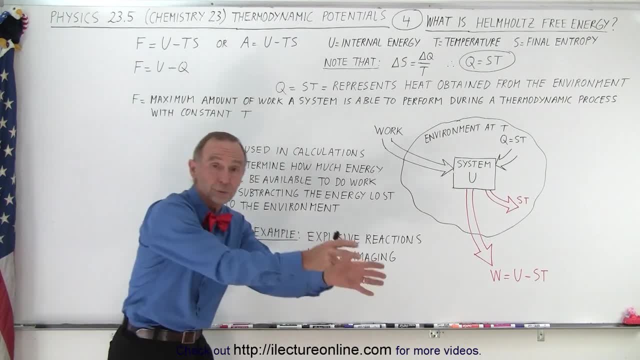 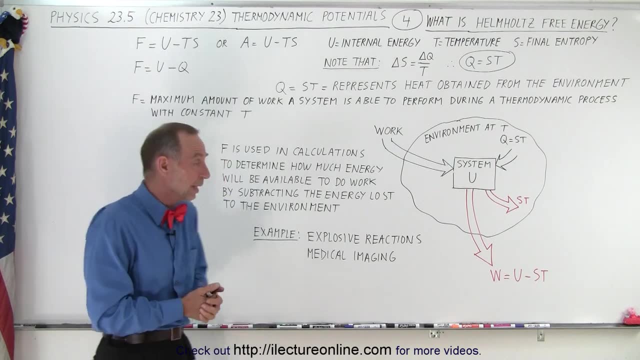 not all of the available energy is really available to do work. Some of it is going to be lost to the environment And it would be good to know how much of it will be used for work and how much of it will be lost to the environment. 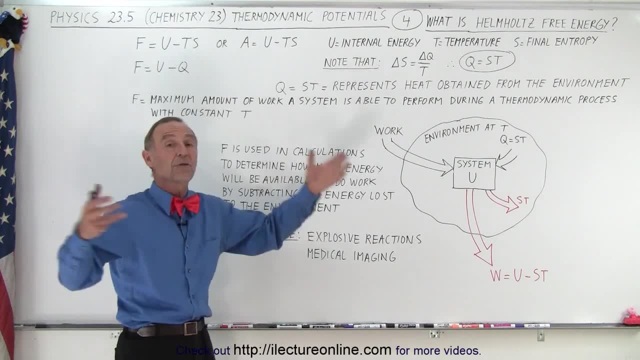 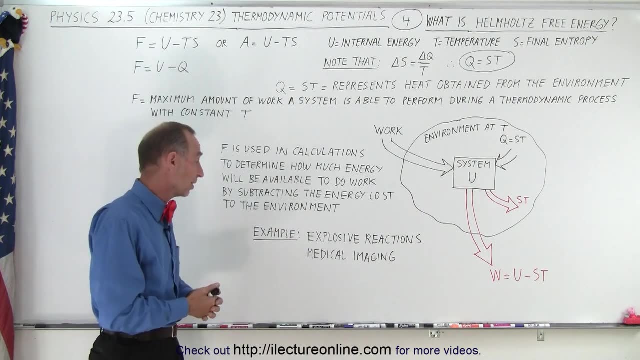 And we can use some examples here- When we have an explosive reaction, how much of the explosion is actually done to do work and how much of the explosion is actually lost to the environment. So that's an example. Or, in medical imaging, not all of the energy of the machine.